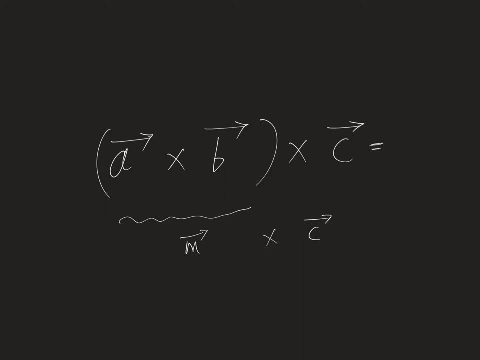 vectors. so, for example, if we take, let's say, M vector is equal to A cross B, then this vector, little m, will be orthogonal to the plane spanned by vector A and vector B. to make it more clear, let's look at an example. in this example we 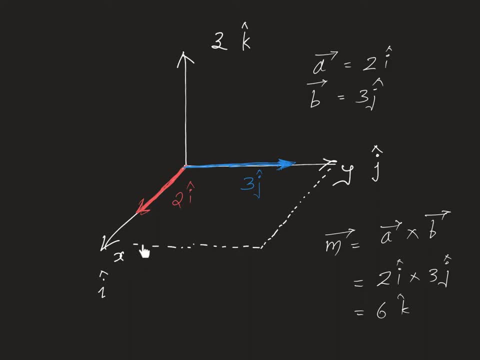 have two vectors: vector A along the x-axis, denoted as 2i cap. then along the y axis, we have 3j cap. this is the second vector B now when I take the cross product of these two vectors, which is fairly easy. so once you do that, 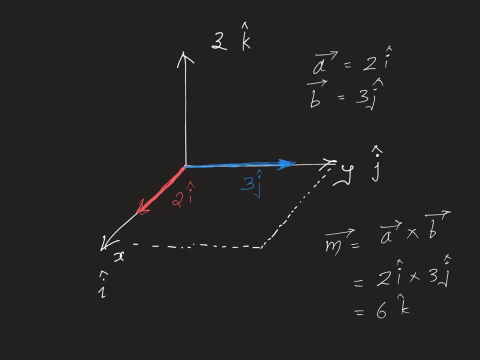 operation you get a vector, 6k cap, so our resulting vector- I will use a different color for that one. so our 6 cap vector will look like something like this, because it is pointing along the k direction or along the z axis and it is having an magnitude of 6. so, as you can see from this illustration that 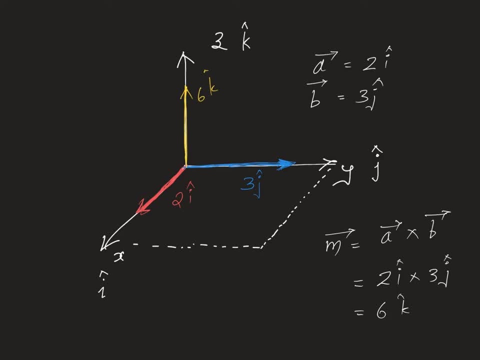 the resulting vector is perpendicular to the plane. xy plane. what is so special about the xy plane? xy plane is spanned by these two vectors. by when I use the words span, what I mean is every vector in this plane. every vector in this plane or can be written as a linear combination of these two vectors or to 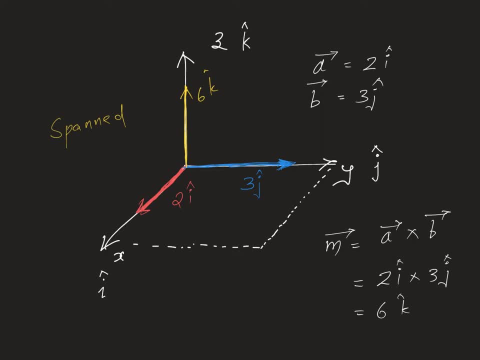 be far more specific. you can say can be written as the linear combination of the unit vectors that point along these two directions. I can tell: take a vector divided by magnitude of a vector will give me the unit vector along that direction. then B vector divided by magnitude of B vector. 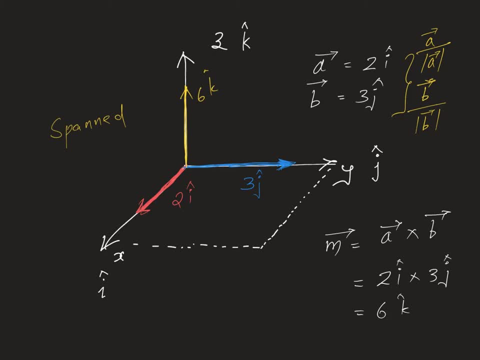 will give me the unit directional vector or the unit vector along vector along the direction of vector B. in a nutshell, this is very easy you have when you take the cross product of two vectors. the resulting vector is perpendicular to the plane spanned by other two vectors, by spanned 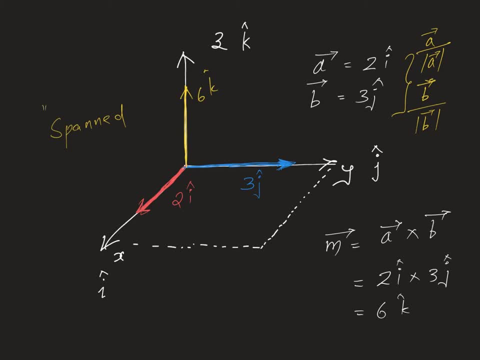 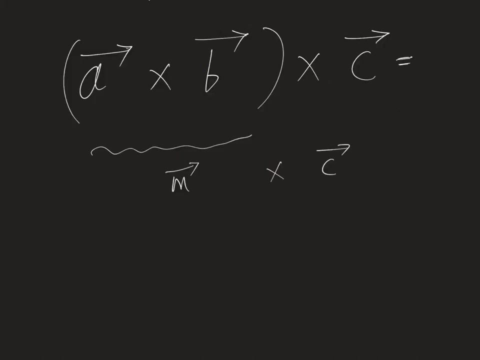 I told you what I mean by the word span. it is very simple. two vectors will always give you a plane, doesn't matter, and this illustration clearly gives you a feel about the result. so I think all of you will agree with me if I say that little m vector is perpendicular to both a and B. now what you can tell. 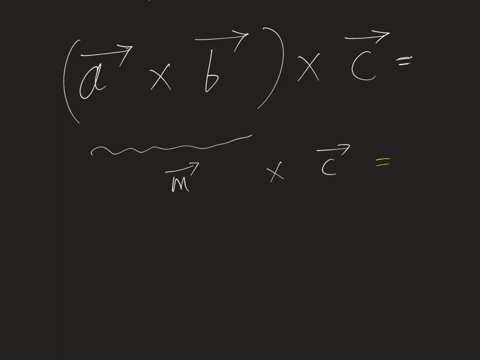 about the right hand side vector. let's call the right hand side vector r vector. now I can tell about r vector that r vector is perpendicular to little m vector, because that's what we just saw. little r vector is perpendicular to our little m vector, which in turn means that r vector lies in the plane. 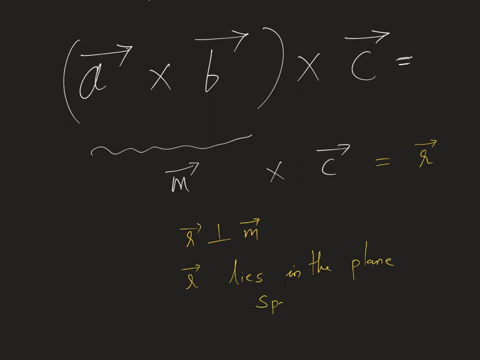 spanned by, spanned by a vector and b vector, make sense. so this is the key concept that you need to understand when you come across vector triple product. since the vector lies in the plane spanned by these two vectors, a vector and b vector, we can write the resulting answer- resultant answer- like this, because it is. 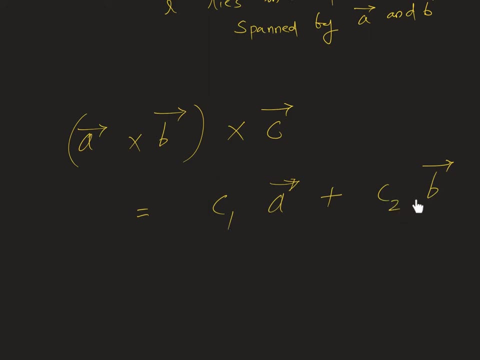 some constant times, a vector time plus some other constant times, the b vector. now everything boils down to evaluating these two constants. i'm not going into those things like how you will evaluate, uh, these two constants and all. now i will write away. i'm going for the. 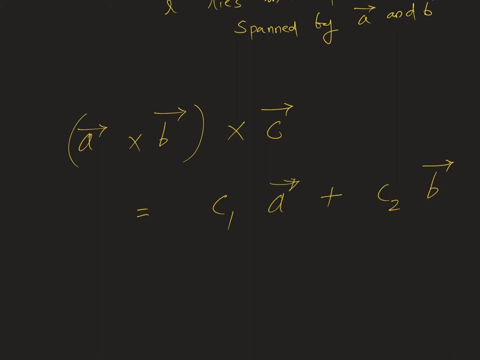 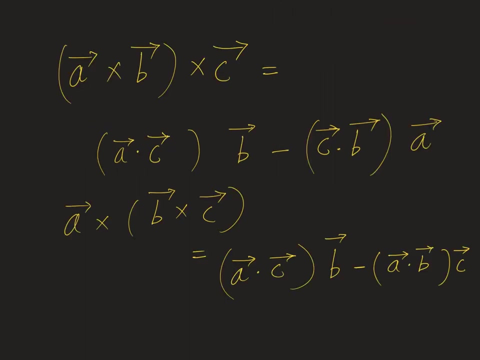 kill. i'm going for, i'm giving you the expressions and then telling you a few tricks to remember that. so these are the final expressions. so the rules goes like this: there are two terms: rule number one, rule number two: there will be always a negative sign for the second term. 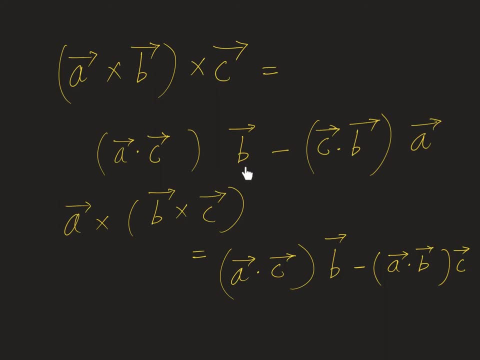 rule number three: the term one will always have the vector which is in the middle of this expression. just to explain rule number three: here the middle vector is b, so the first term has vector b in it. here again, the middle term is b and the first term has. 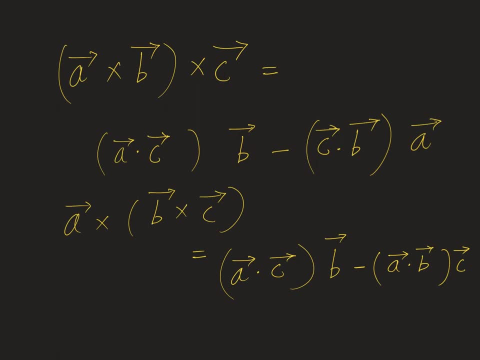 vector b in it. so rule number three one was there are two terms. rule number two: there is always a negative sign with the second term. rule number three: middle vector will be always there in the first term. it is not there as a dot product is there as it is make sense, then things are fairly easy. because once you know that, 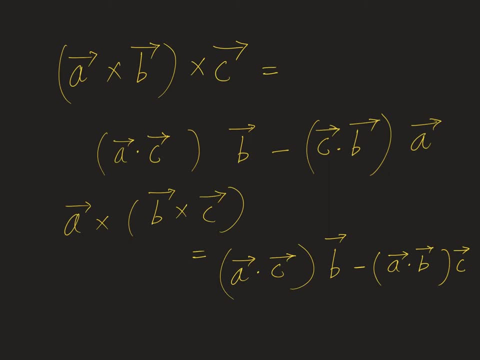 the middle vector is there in the first term. you know this resultant vector is in the plane spanned by a vector and b vector. so once you have b vector here, then in the second time you should have your a vector. but when you come to this expression you know that the resulting vector 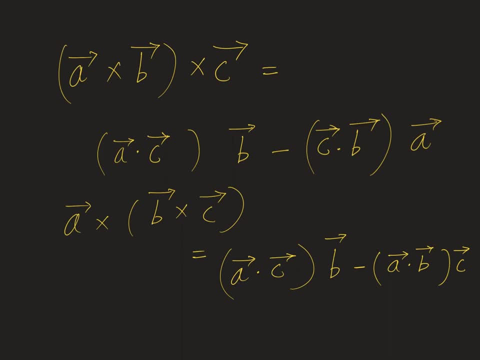 as per this expression lies in a plane spanned by these two vectors, vector b and vector c. because if vector b and vector b- sorry, if vector b cross c, is some vector. let's call it. i'm running out of alphabets here. let's say n cap, so the resulting vector should be perpendicular to n cap. 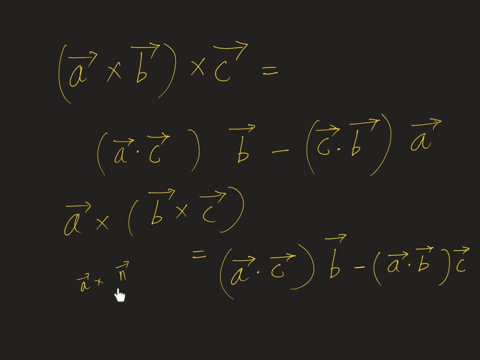 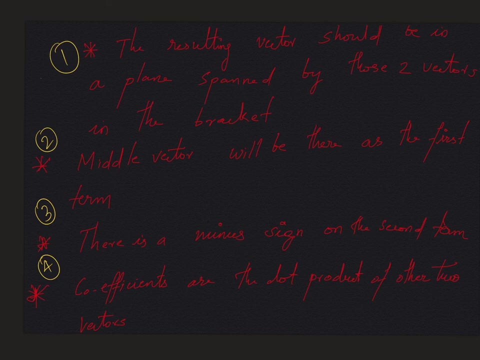 makes sense, which in turn means that the resulting vector should lie in the plane spanned by vector b and vector c. so let me summarize all the things, what we have discussed. i have written here one after the other. the resulting vector should be in a plane spanned by those two vectors which are in the bracket. then middle vector will be there in the 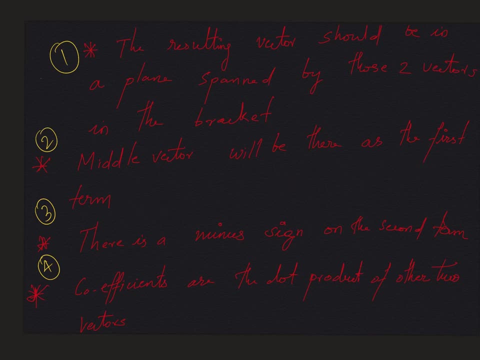 first term, the middle vector, the b vector. in the two above examples there is a minus sign. on the second term, then, coefficients are the dot product of other two vectors. so with this intuitive understanding i think you will never have to memorize the formula for vector triple product. thanks for watching.